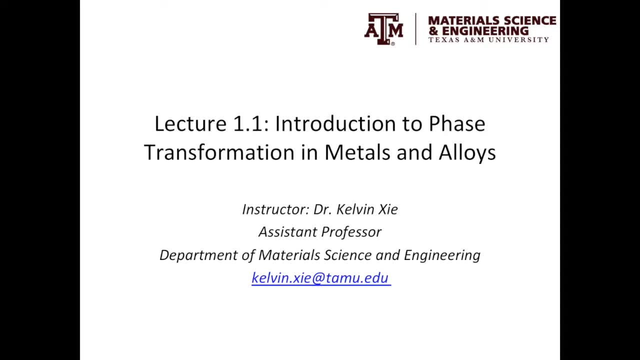 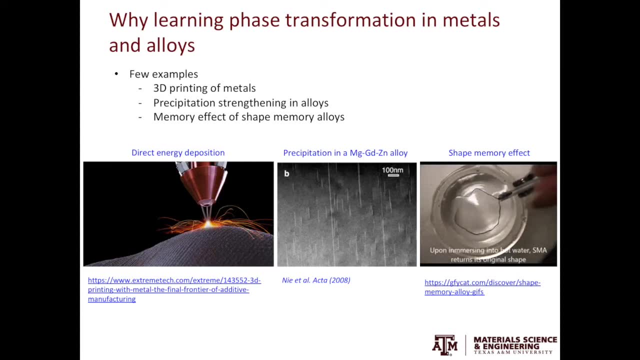 Howdy. In this new video series, we're going to discuss the phase transformation in metals and alloys. Let's start by asking ourselves why we want to learn phase transformation in metals and alloys. Here are three examples. The first example is metal 3D printing. More specifically, this technique. 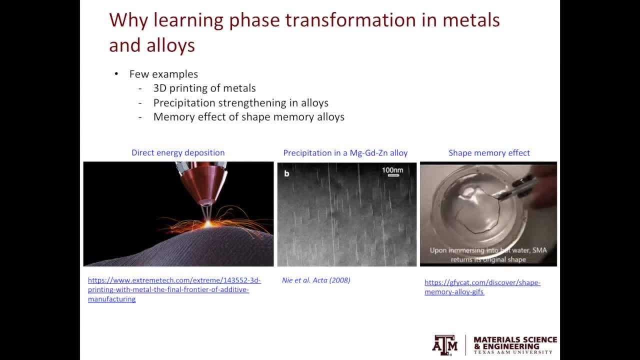 is called direct energy deposition. When doing printing, the metal particles are sprayed on the surface. Meanwhile, either a high energy laser beam or electron beam were used to melt those metal powder particles. The molten metal pools then solidifies and turns into part of the printed. 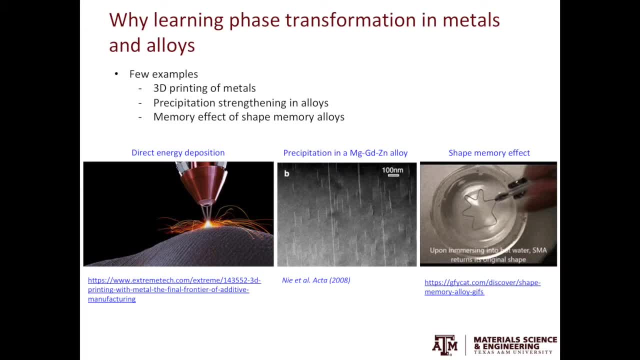 components. So, as you can see, this is a good example of the liquid to solid transformation in metals and alloys. The second example is precipitate strengthening in alloys. For those who have taken undergrad levels level material science, you know that growing precipitates is an effective strategy to increase. 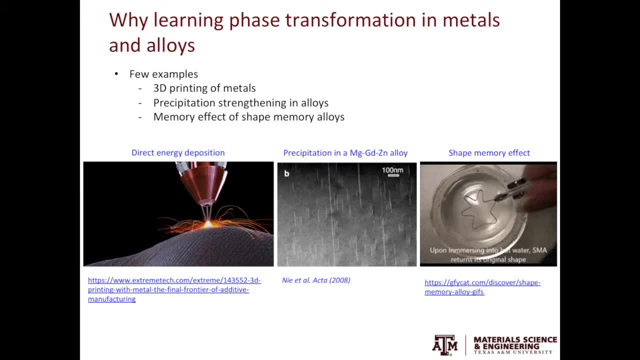 the strength or hardness of a material. The process how these precipitates grow is also a part of phase transformation, which is a solid to solid phase transformation. The bright features you see in the micrograph in the middle, these are the nanoscale precipitates. 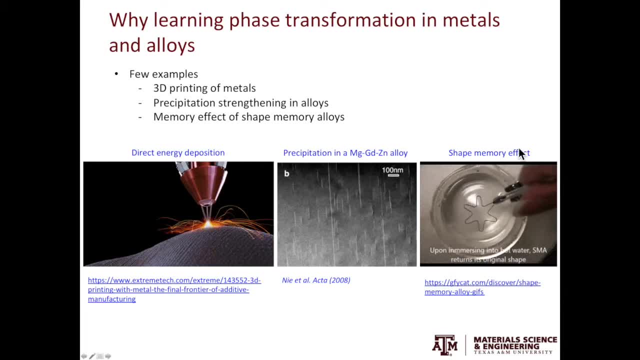 The third example is shape memory effect in shape memory alloys. If you plastically deform the shape memory alloy, then put it back in some hot water. it will spring back to the original shape. The ability to remember and to restore to the original shape in shape memory alloys. 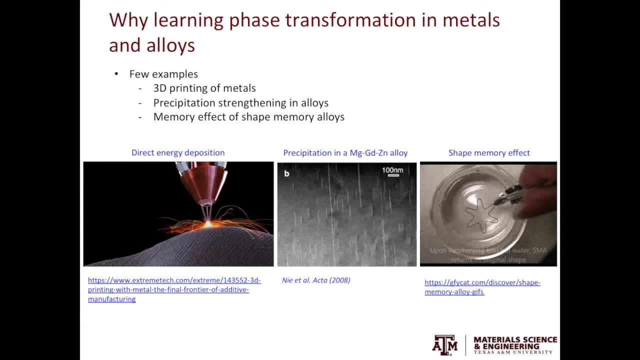 is also governed by solid phase phase transformation, and the process is called martensitic transformation. Let's come back to the question we asked at the very beginning of this slide Why we want to learn phase transformation in metals and alloys. This is because the knowledge are widely used in alloy design and development. 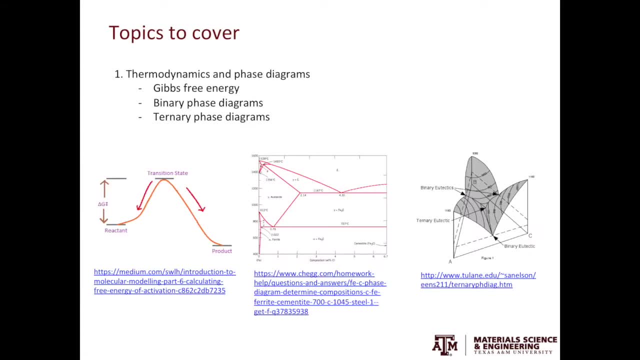 There are five parts in total in this video series. The first part is basic thermodynamics and phase diagrams. In this part we'll discuss Gibbs free energy. Gibbs free energy really governs any types of chemical reactions or phase transformations. Then we'll discuss binary phase diagram. 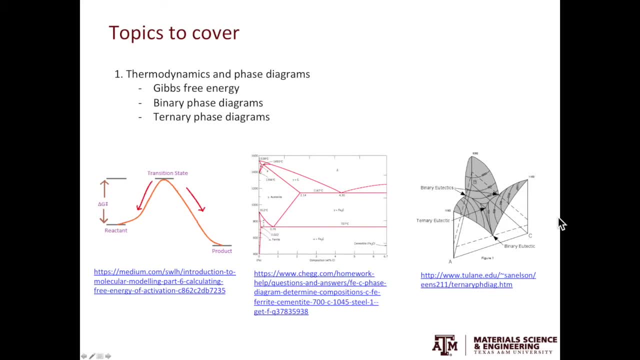 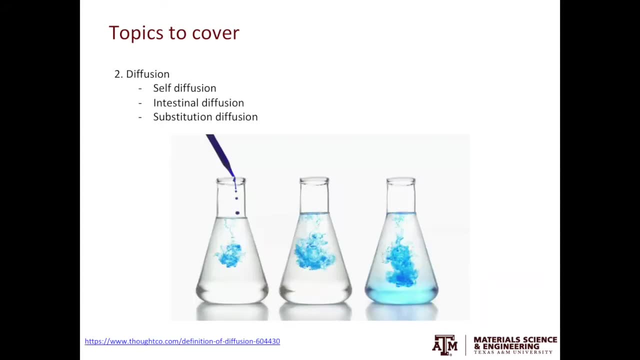 The example is iron carbon phase diagram. then we'll move to ternary phase diagrams. The second part is diffusion. In the example here, if you put a few drops of ink in clear water, the ink will diffuse out and this process is diffusion. 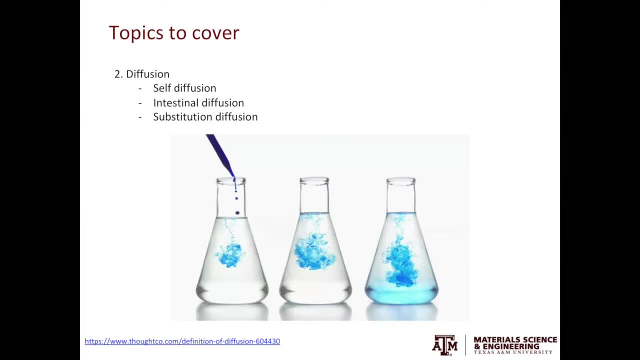 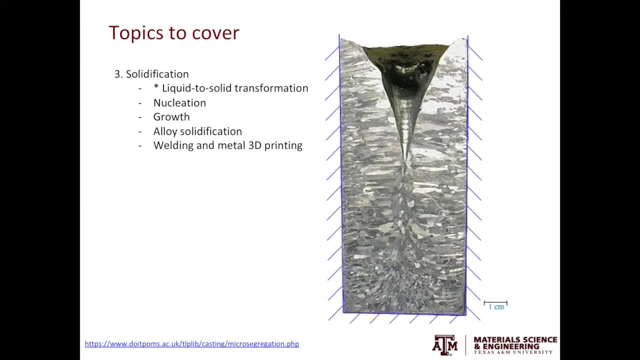 In this part we'll discuss self-diffusion, interstitial diffusion and substitutional diffusion. In the third part we'll discuss solidification. Solidification is a liquid to solid transformation. In details, we'll describe nucleation growth, alloy solidification, welding and metal 3D. 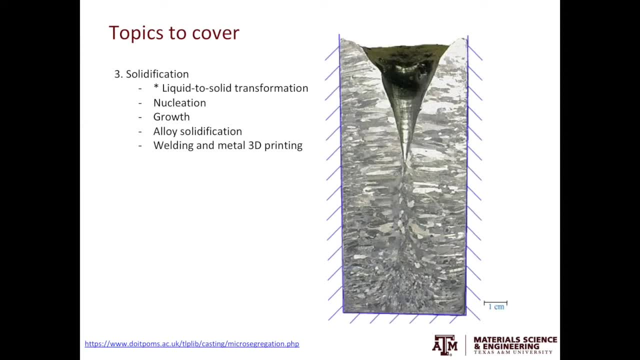 printing. Here is a teaser. This is a cross-section of some solidified metal. If you have a closer inspection, the microstructure near the surface looks quite different from the microstructure within the material. The grains near the surface are solidified. 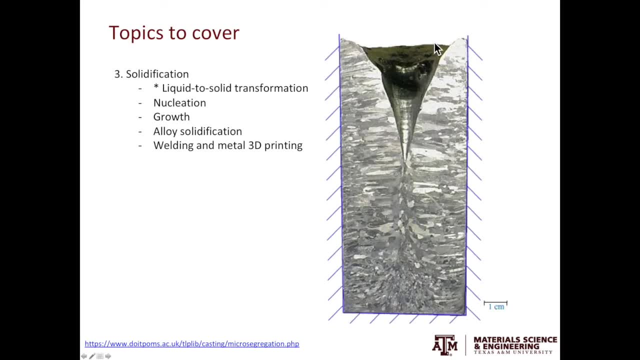 The grains near the surface are solidified. If you have a closer inspection, the microstructure near the surface looks quite different from the microstructure in the material. The grains near the surface are solidified. The grains near the surface are solidified. 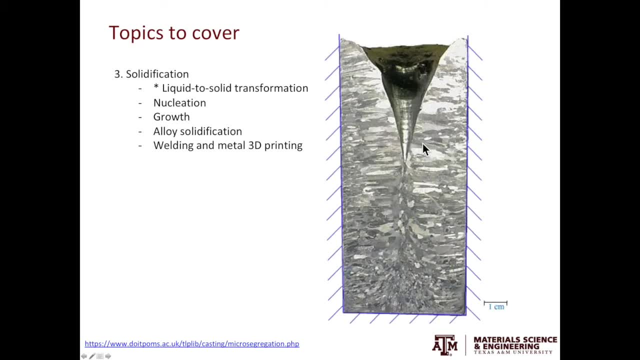 If you have a closer inspection, the microstructure near the surface looks quite different from the microstructure in the material. This is a cross-section of solidification. If you have a closer inspection, the бы a solidification. If you have a closer inspection, the be a solidification. 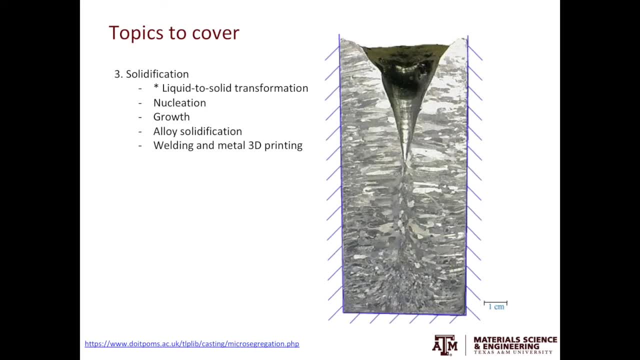 At least 90% of solidification is solid. Highly diluted solutions are much smaller and equiaxed in morphology, while the grains near the centre are elongated. Why this is the case? You will find the answer in one of the future videos. 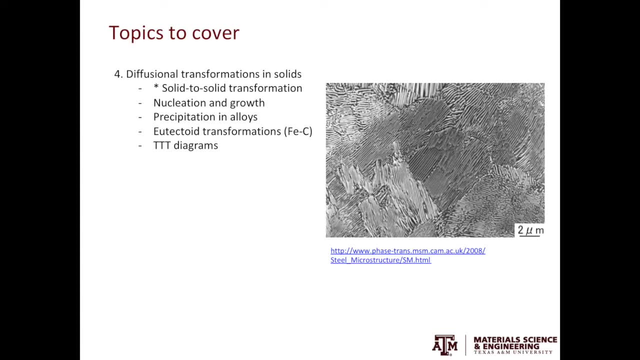 The fourth part is diffusional transformation in solids. Unlike solidification, which is liquid to solid transformation, diffusional transformation is solid to solid transformation. Here we'll also discuss nucleation and growth, followed by three examples: precipitation in alloys, eutectoid transformations and the time-temperature transformation diagrams. 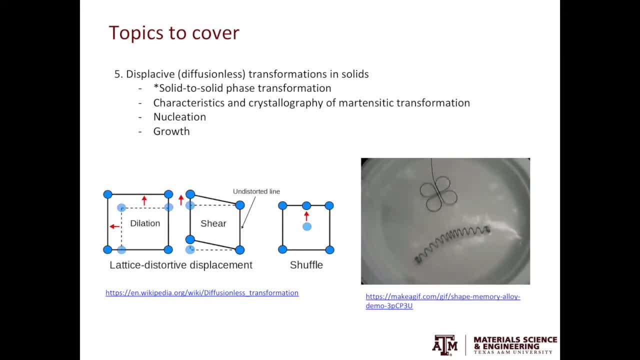 Last, not the least, is the displacive transformation in solids. There's no diffusion involved in displacement transformation. that's why it's also called diffusionous transformation. Again, it is solid-to-solid phase transformation. The atomic repositioning are mediated by either dilation, shear or shuffle, and there's no diffusion involved. 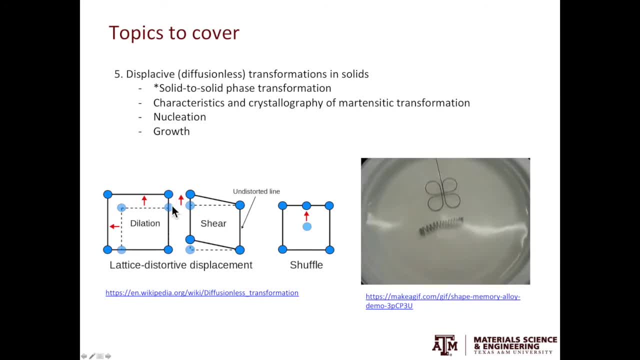 The atomic displacement is less than one unit cell, whereas in diffusional transformation atoms can move much, much larger distances. Again, displacive transformation is also a type of solid-to-solid phase transformation. We'll discuss characteristics and the crystallography of modern silicon.